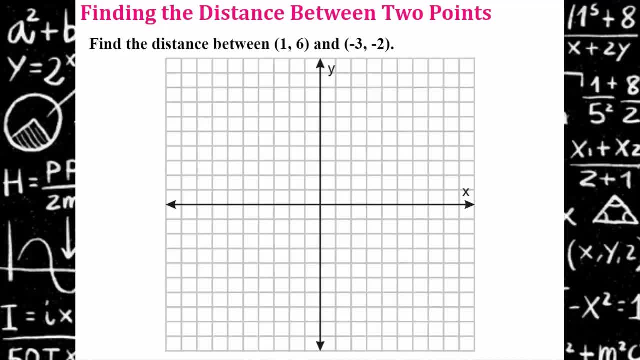 example, We're going to go through those four steps to find the distance between these two points. So step one is to plot the two points on the coordinate plane. So here I've plotted one six and negative three, negative two. Step two: draw a line segment to connect the two points. 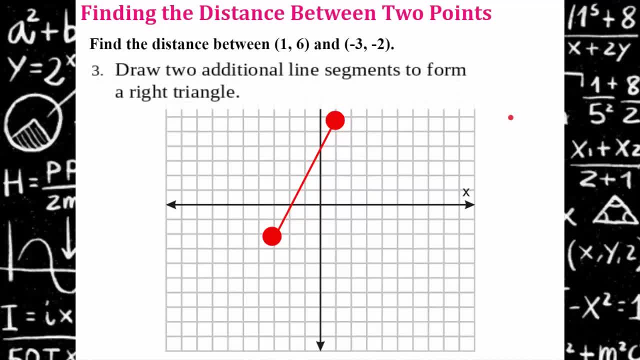 Step three: draw two additional line segments to form a right triangle. Part of that step. you want to find the units of the measurement of the two legs, So one, two, three, four, five, six, seven, eight units for this leg and four units for the smaller leg. 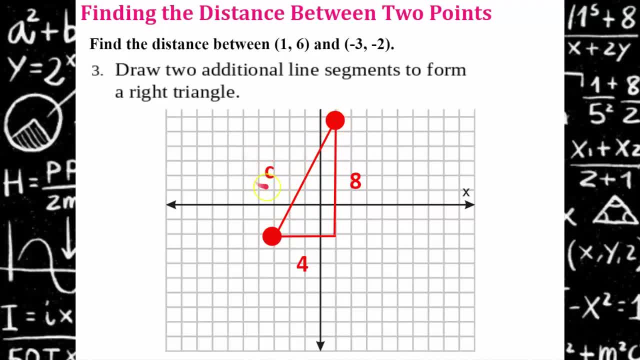 This diagonal line that we're trying to find the length of is my hypotenuse c. Step four: we want to calculate the distance of the hypotenuse using the Pythagorean theorem, which is a squared plus b squared equals c squared. Evaluate for the values of the legs four and eight. 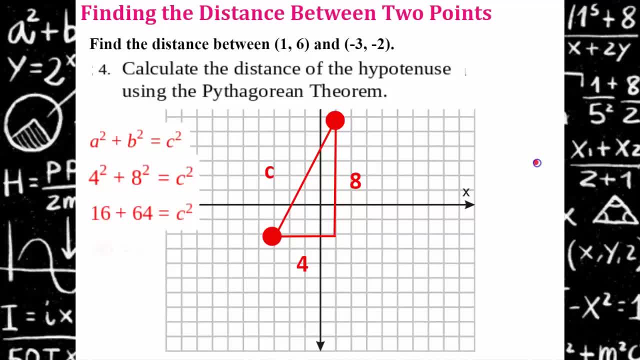 Do the math: Four squared is 16 plus eight squared is 64.. Add 16 and 64 to get 80.. Take the square root of both sides and see. my hypotenuse is equal to 8.9 units Traditionally. 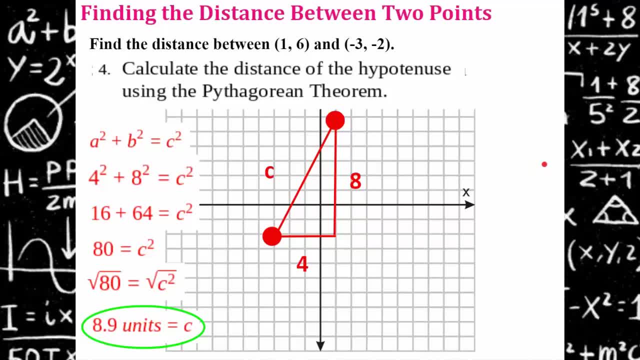 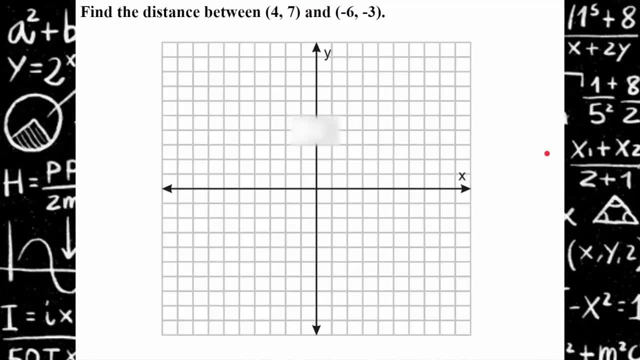 you're going to round to the nearest tenth, unless the instructions tell you to do something else. So go ahead and pause the video now and see if you can find the distance between these two points. When you have found the answer, please hit play and check your answer. 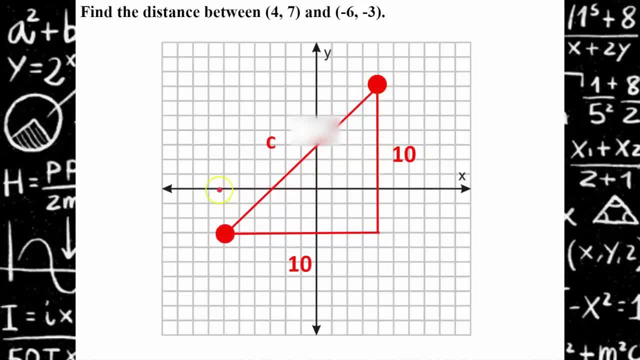 So here I've plotted four, seven and negative six, negative three. I found the length of both legs, which is 10 and 10, and I'm looking for that diagonal distance c, the hypotenuse. So I use the Pythagorean theorem. I evaluate with the legs a and b. both are 10,. 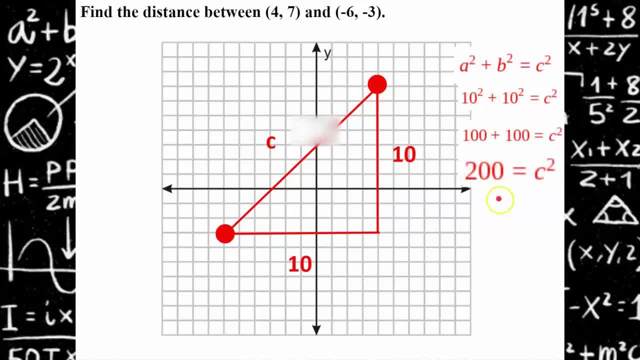 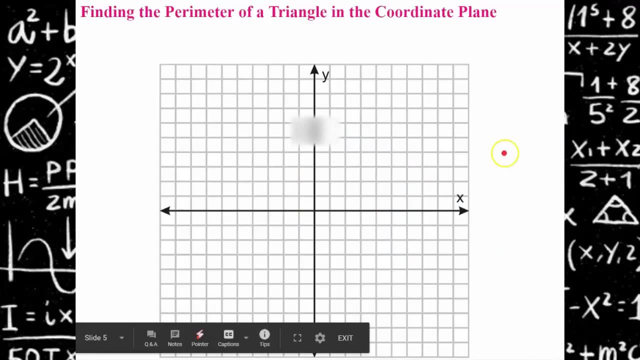 10 squared is 100, so 100 plus 100 is c squared. c squared equals 200.. Take the square root of both sides. The square root of 200 is 14.1 units when rounded to the nearest tenth. All right, so now we can also use this to find the perimeter of a triangle in the coordinate plane.